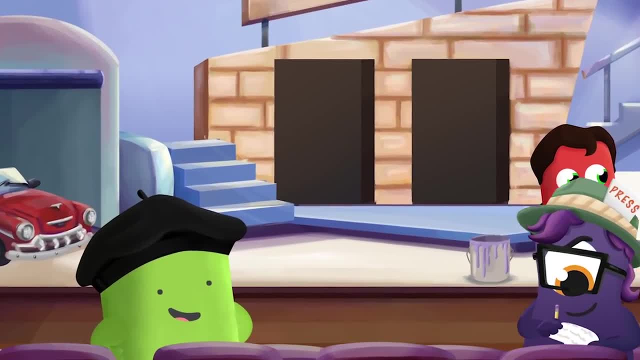 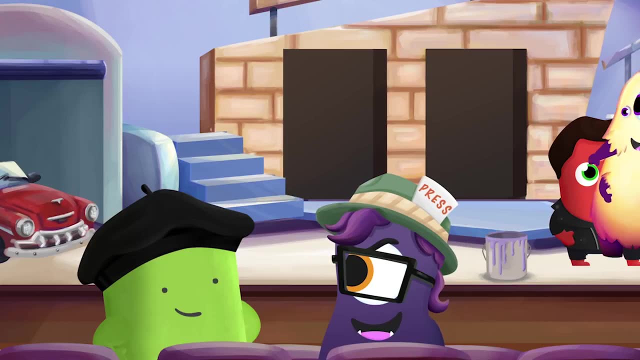 Just then, Maya from the school paper stopped by to see how the play was going. Excuse me, Mojo, Maya here from the Monster Herald. Four days until opening night. Will your team be ready? I think so, said Mojo. I think so, said Mojo. 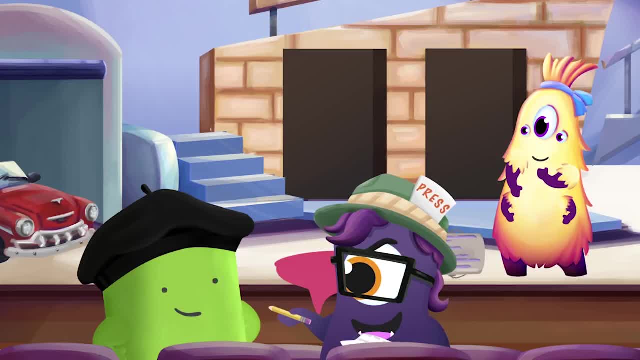 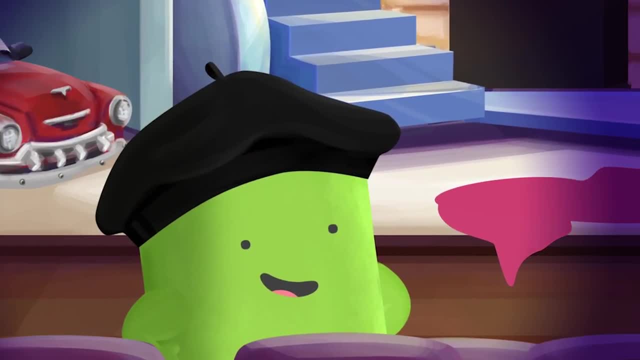 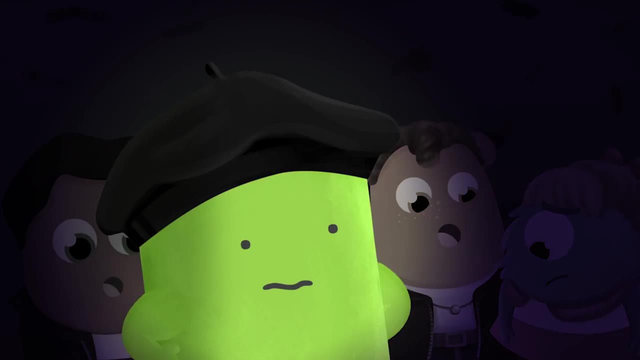 I think. so said Maya. We're all working really hard. Well said, Maya. I just hope you don't embarrass yourselves. Thanks for your time. For the first time, Mojo began to feel anxious about the play. Did he set his friends and himself up for total failure? 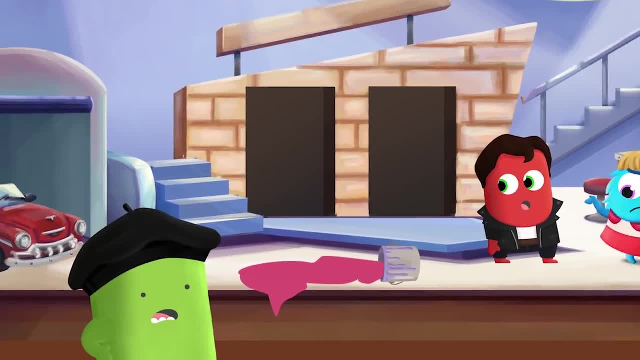 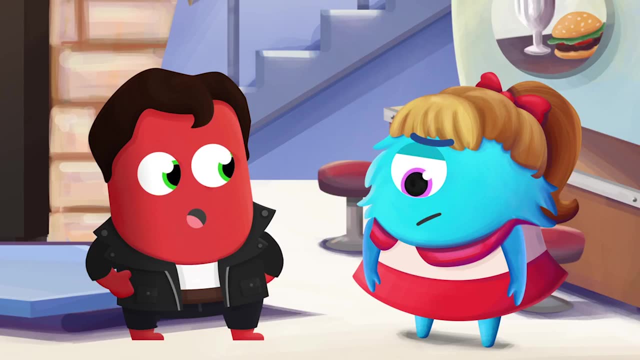 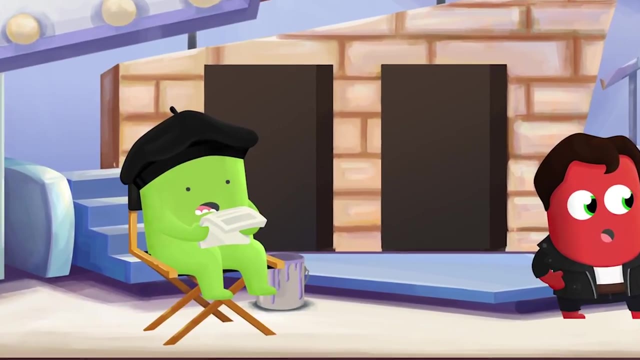 He suddenly snapped at Katie Katie. study the script tonight, said Mojo, Don't forget Katie Katie, Katie, Katie, Katie, Katie At the next day's rehearsal. as he read the school paper, a strange feeling of anxiety. 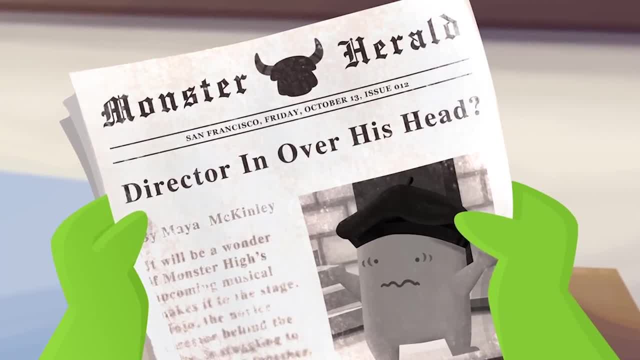 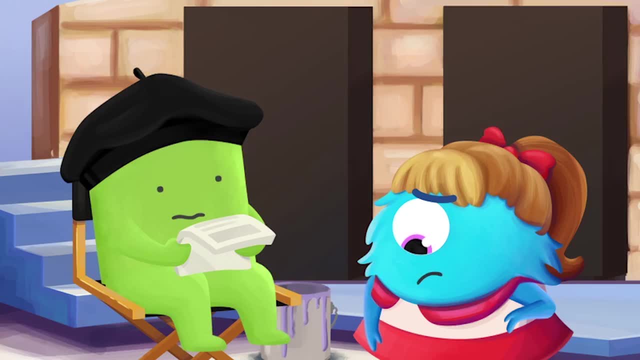 grew inside Mojo. Mojo said: Katie, I can't remember this line. Can you help me? In a split second, the anxious feeling rapidly grew. Mojo began to sweat. He was suddenly furious. Do any of you even care about the play? 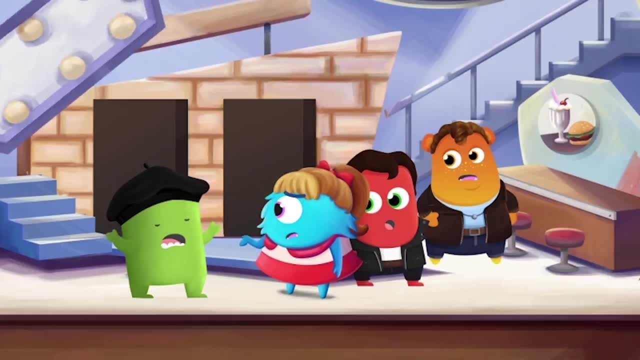 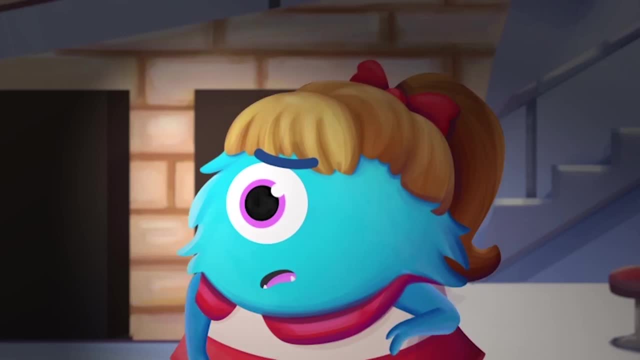 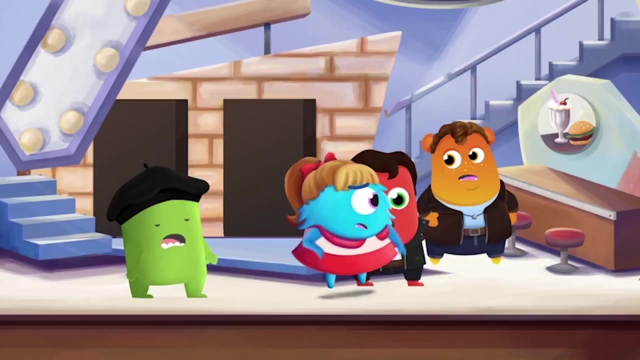 He yelled. There was silence on the set. Katie, he said, I never should have let you be in my play. You don't think I'm trying, said Katie. Fine, you can do it yourself, because I quit. Katie rushed off the stage. 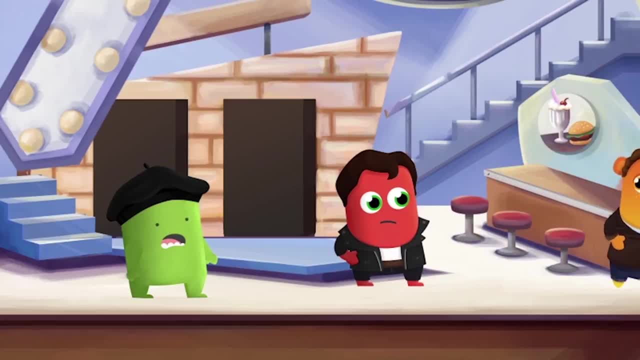 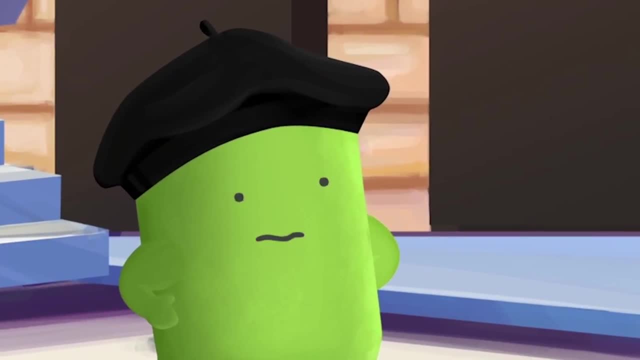 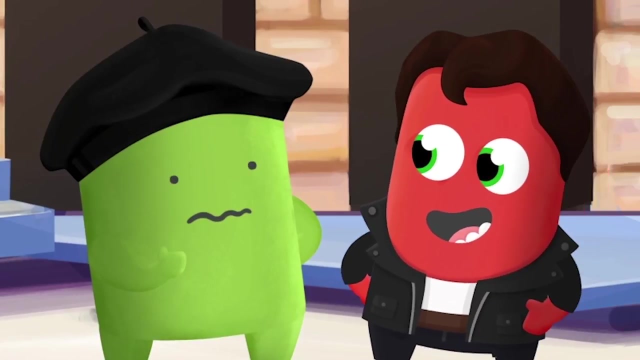 The other monsters followed. No one wanted to work with Mojo And he was acting like this. Mojo's fury turned to a panic. Opening night was only three days away and his own friends had walked off set. Green Man said: Bruce, I've got some friends you should meet, but we've got to move quickly. 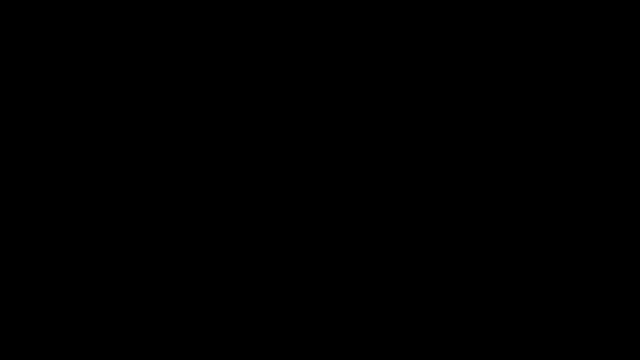 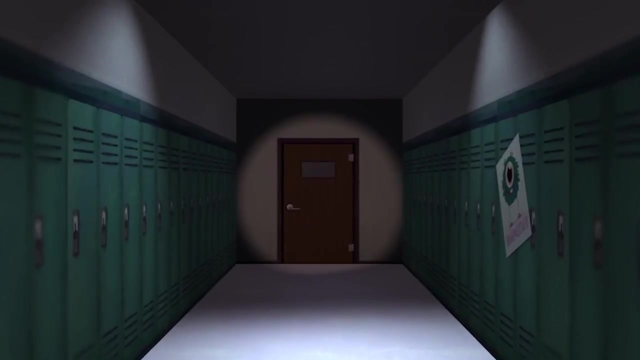